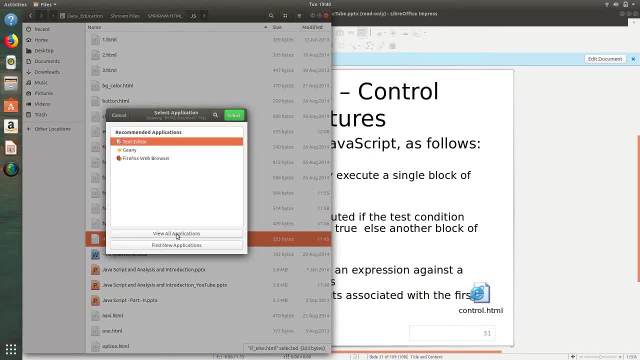 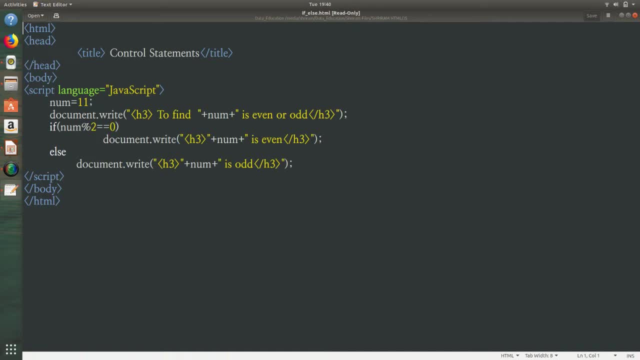 So I am going to just open the switch, I mean, if else right now, so you can see that here. so it is control statement. you can see that. exactly the same code, whatever we have typed for HTML. I am following the same tags and same syntaxes, but inside script I am including my javascript. 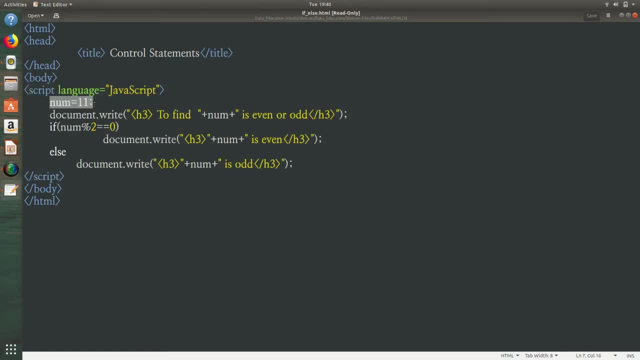 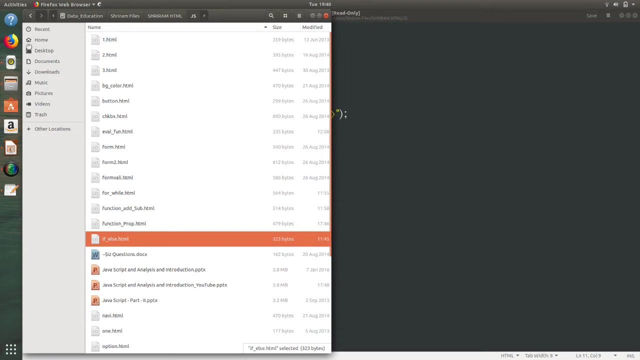 Now see, here I have got a number equal to 11,, num equal to 11,. now I am going to find if it is odd. or even so, how do you find it? if number mod 2 equal to 0,, then it is. even else it is odd. very simple. so I am going to run this code right now and you can see this. see the way I have used the syntax here. if else, it is exactly the same as whatever we have used in our C programming and I am going to just run it right now for you here. 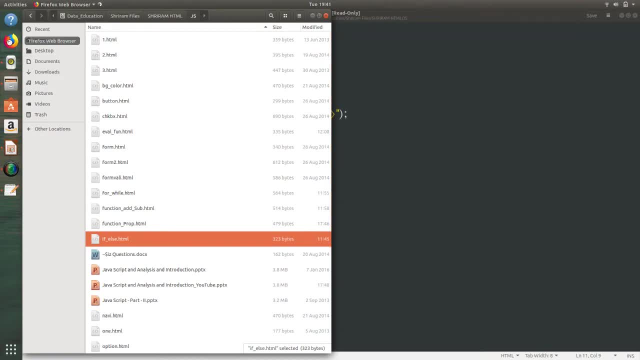 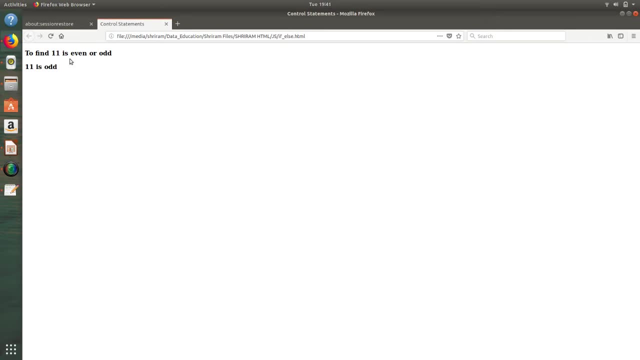 So you can see the result right now in front of you, maybe in half a second- it takes a little longer than expected- so you can see that to find 11 is even or odd, 11 is odd. so the result has come right now in front of you and this is how it works. so, if else is as similar to whatever you have learnt in your C programming, there is no change. 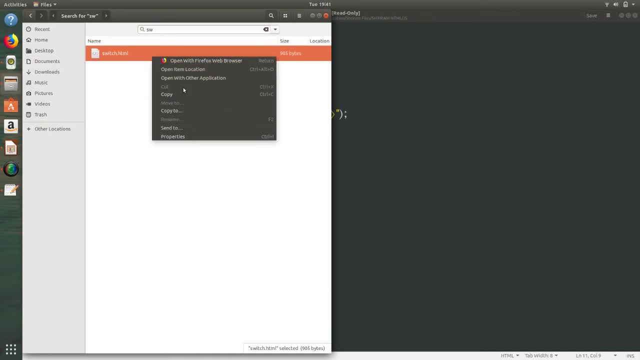 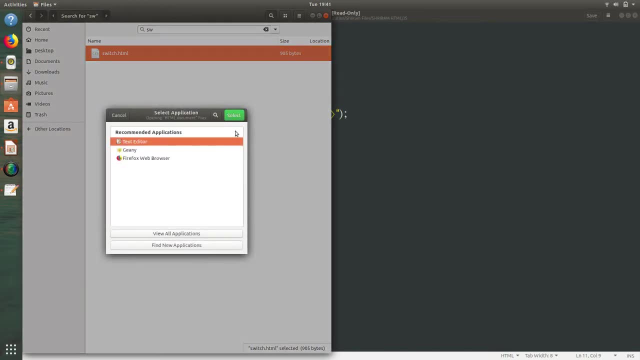 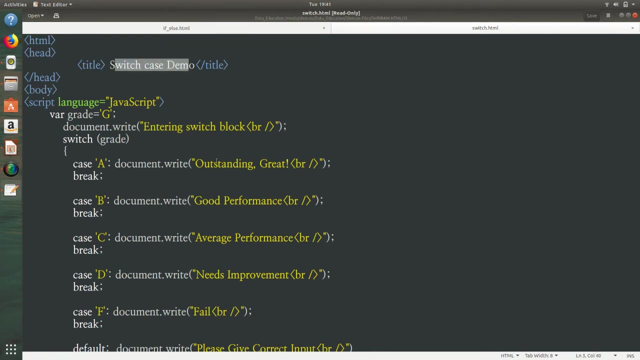 Now our time is to learn. now we need to learn this Switch case and it is again similar to whatever we have learnt earlier, so I am just going to show you the code. I am having a switch case demo as the title. I will show you where it comes also. now what I am going to do is I am going to have the grade entered here where grade equal to G, switch grade. so this grade is coming here and now. if grade is A outstanding, if grade is B, it is good performance. if grade is C, it is average performance. if grade is D, it is average performance. 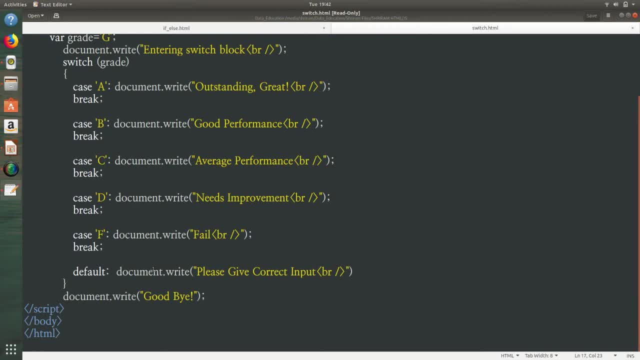 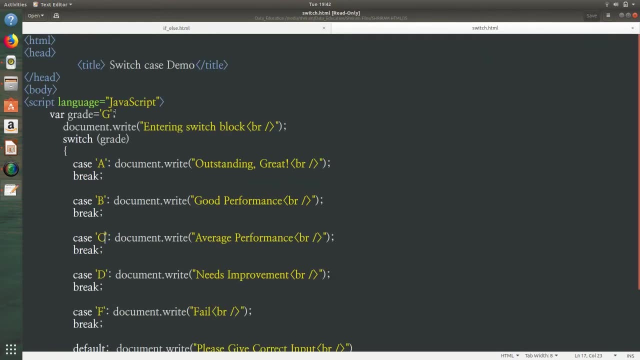 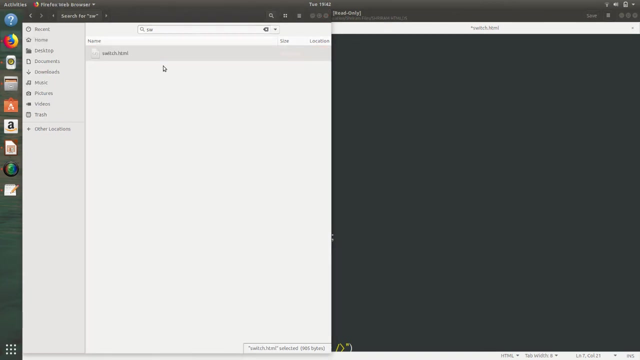 It needs improvement. if it is F, it is fail. if none of these options are there, it is as good as C and you need to go with the default option. so I have given an option called as G. here. I am going to change it as A now. next time I will show you how exactly to run it as G. I have saved it now I am going to run it. so this is a simple switch case demo. so you can see that right now in the Firefox browser, whatever I am going to open right here. so entering the switch block, please give the correct input because I have not saved the correct input. so please give the correct input because I have not saved the correct input. please give the correct input. 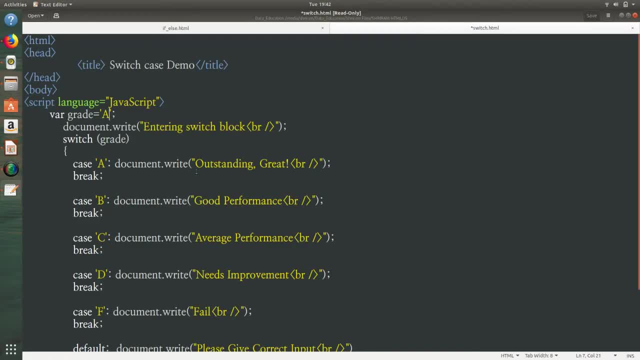 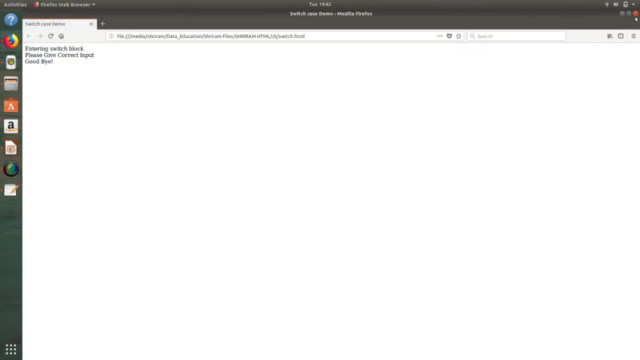 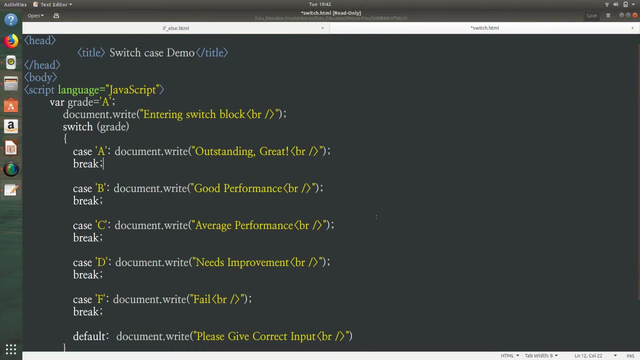 it? i think so. i need to save this code, then when i do it it will probably be updated properly. so i am doing an fi here once again. i have. i need to just save this file, which i have not done. so switch case is here. oh, this has got a rewrite permission problem, so i have done it in windows. 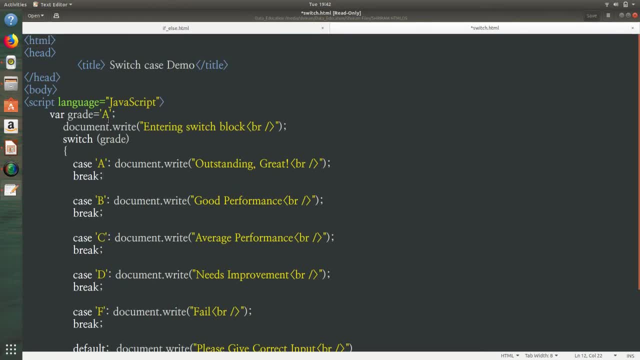 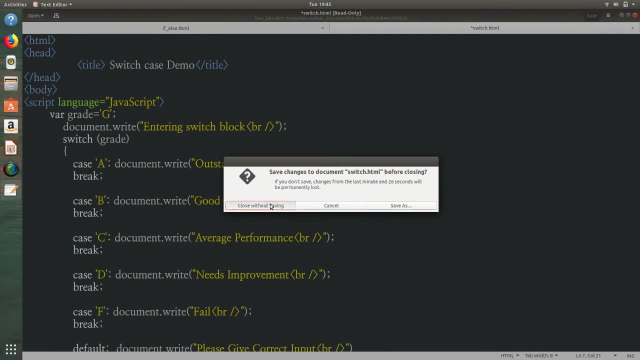 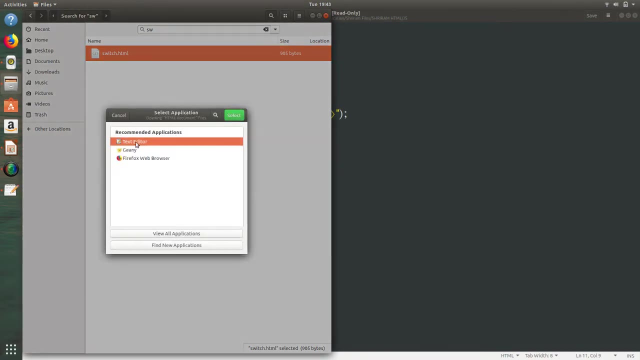 and now i need to edit it with proper permission. so now let us retain it as g alone. so when you see it as g, you will see that when i am closing it i will open it again so that you can understand it better. close without saving: i am opening it again. you can see that now i am having the same. 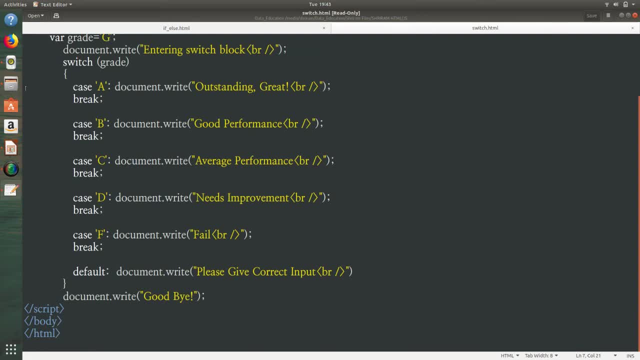 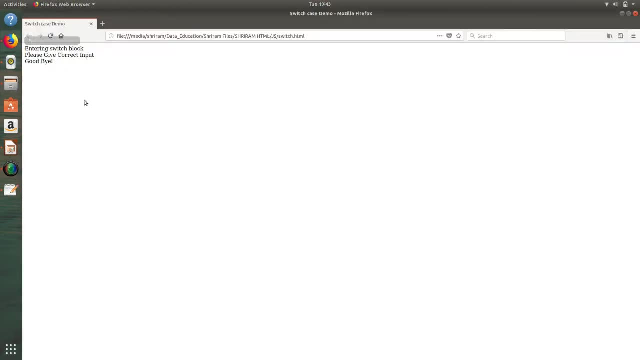 contact. it is g. g means it should go to the default option, so i will now run it. um, i do not have the edit permission here, so i am running it so you can see that i have got an output. please give the correct input, which means g is not the right option that i have to give, so there is a. 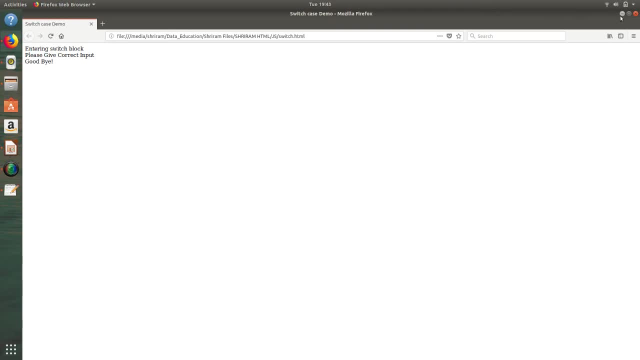 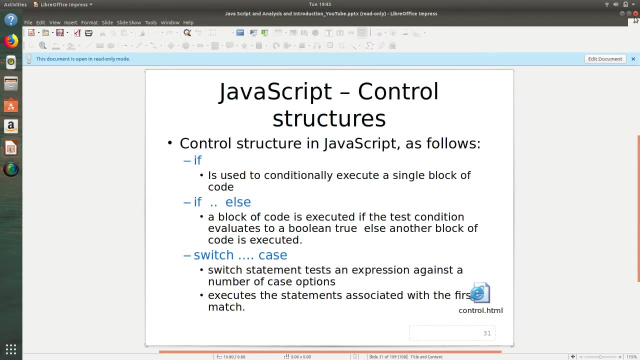 d default option, which is being picked up. it is exactly like c programming. there is no major difference here in this case. i hope you guys understood this. um, if you have any doubts about it, you can probably ping me. we will go to the next one quickly. uh, the next one is going to be a while. 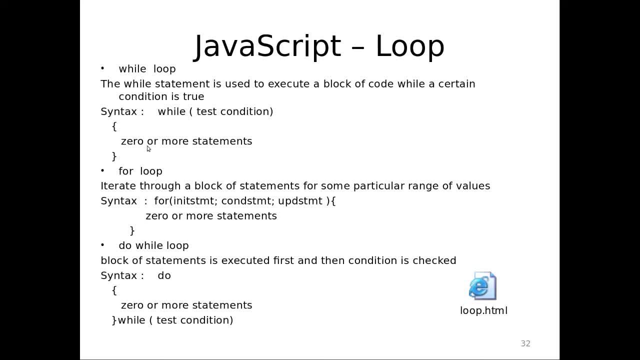 loop and for loop. while the condition is true, it will go and execute the statements inside the block. similarly, for i equal to 0, i less than 10, i plus it is as good as c. there is no change. so if there is no c programming's for loop, there is no difference. so i am going to use the same for loop. 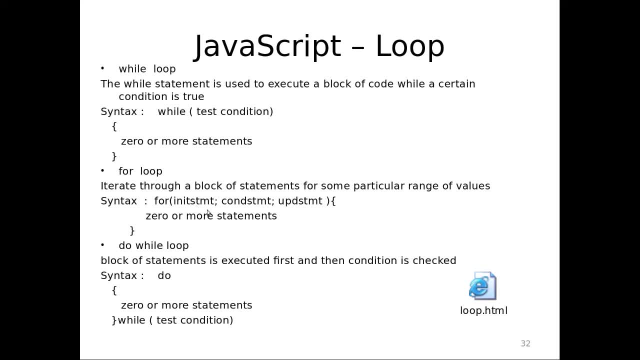 here. so here i am going to instantiate- i mean initiate- i will check the condition and i will do the action. i will initiate, check the condition, go to the, go to the content of the loop, then update the value here. so it is as good as c programming. there is no major difference here. so let me see an. 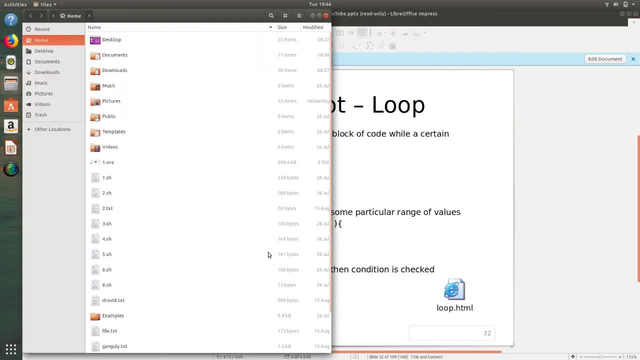 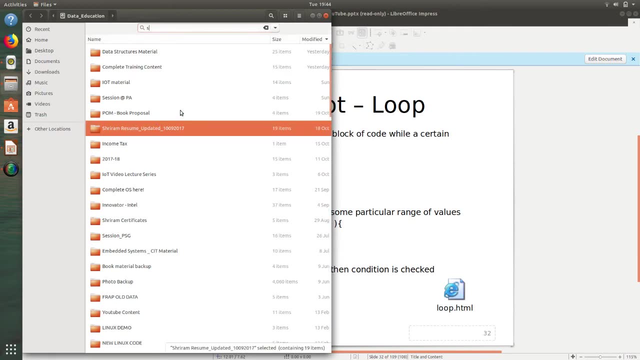 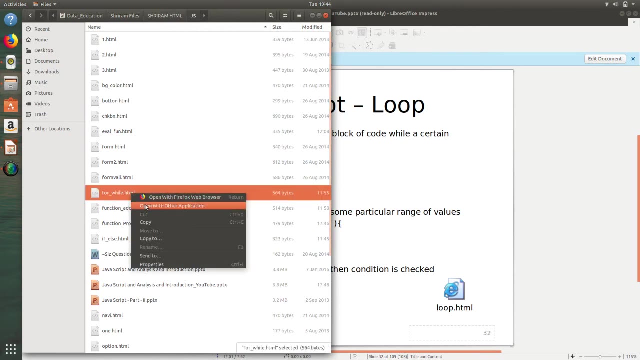 example. let me show you an example which will probably make your understanding a little better. i am going to show you a very simple example that will help you understand uh things better. so, once again, and yeah, i have it here right now, so it is for loop and while loop, so i am going to 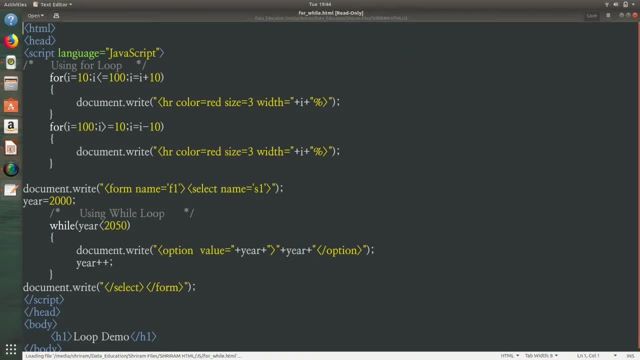 open a text editor with the content. now you can see that here. so i have got a for loop. i am going to design some pattern. i am going to show you some pattern. so for that i have used for loop for i equal to 0, i less than 100, i equal to i plus 10. then it will come here. one side i will keep. 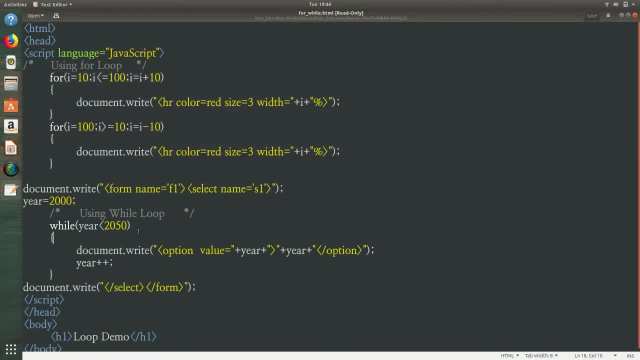 incrementing another side. i will keep decrementing. and also i have i got something called as here. i have got a variable called as here, while here less than 2050. i'll keep a box here, so simple, so don't worry about. uh, what is it? why do we do it? i'm just 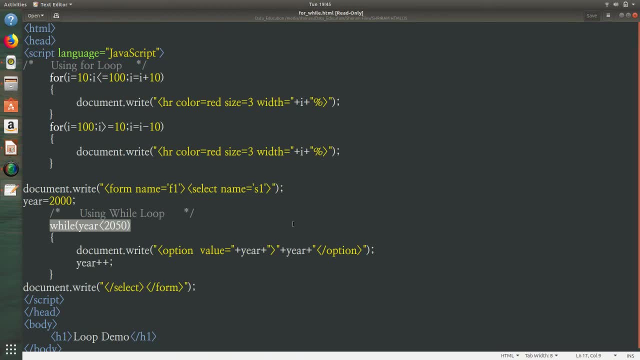 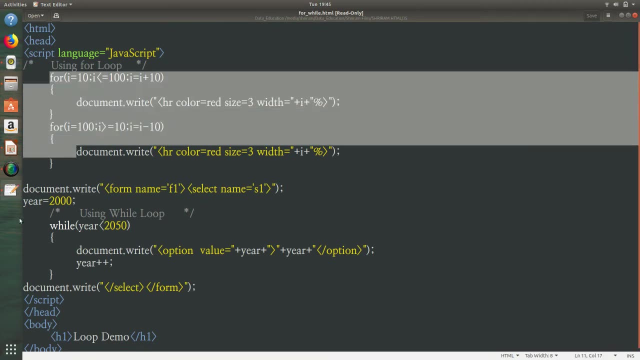 showing you the usage of the loop here. you can see that i have used while loop here like this. i have used for loop here like this. i am going to now show you the output so that you can understand how exactly this one worked. what is this form? and other things we will see later, don't worry. 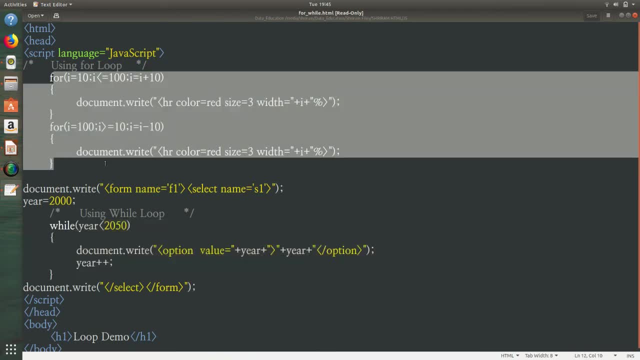 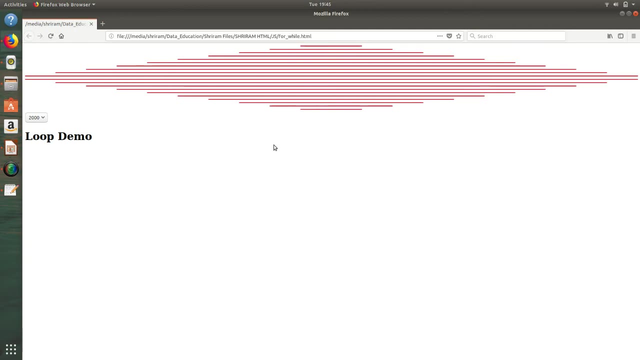 about it. i have embedded the while and far in one code so that you can see the output and the syntax and understand it easily now. now i am opening it in the browser so you can see that here. this is the pattern that i have generated because it should be incrementally working here. 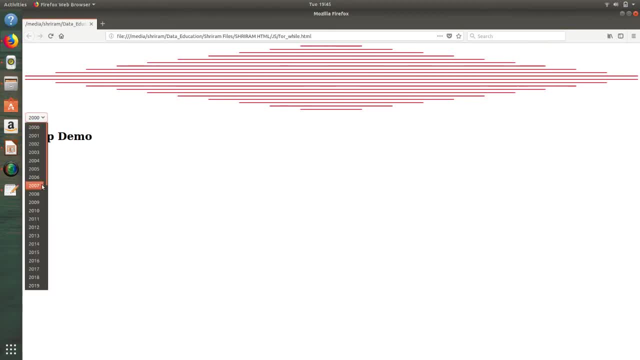 and then it has decremental here. it has decrementally come down here and till 2050 is what i have got it in the box. so this is a simple example that i can show you. for while loop and for loop, the syntax is pretty much similar to whatever we have learned in c programming. 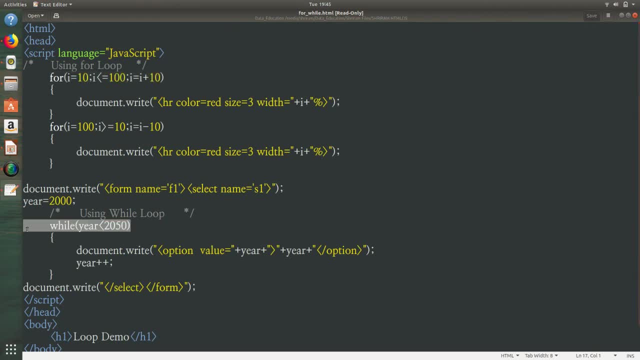 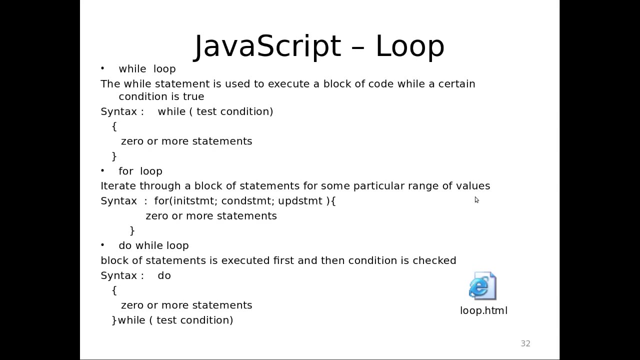 remember it, there is no difference. so the syntax for do while while for everything is the same and there is no major difference with respect to these three syntaxes, and i hope the example that i have given you is sufficient for you to understand how it works. this is what i example i have given you.